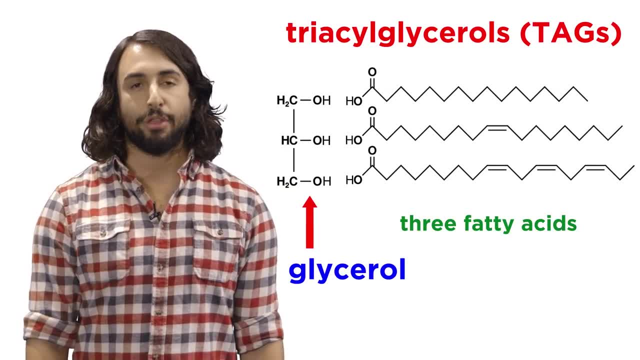 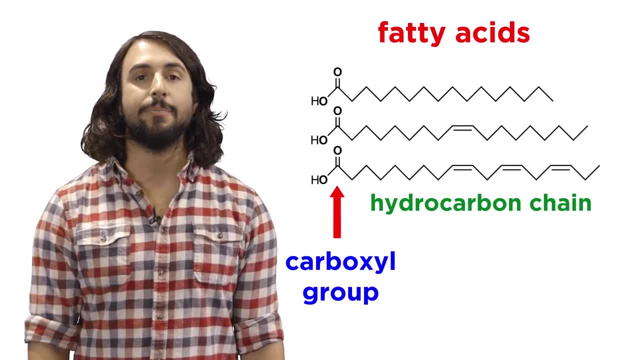 off this portion of the molecule we get glycerol and three fatty acids. They're called fatty acids because they are carboxylic acids, but they also have long nonpolar hydrocarbon tails which can vary depending on the TAG the fatty acid is derived. 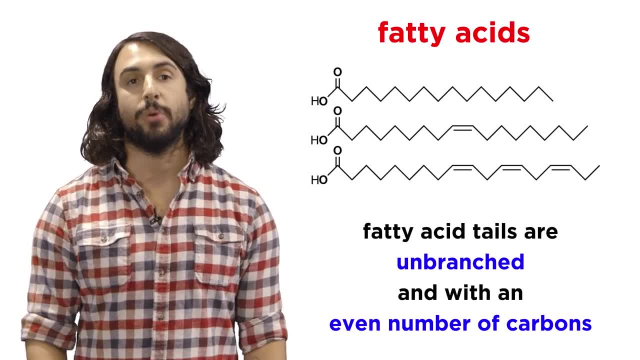 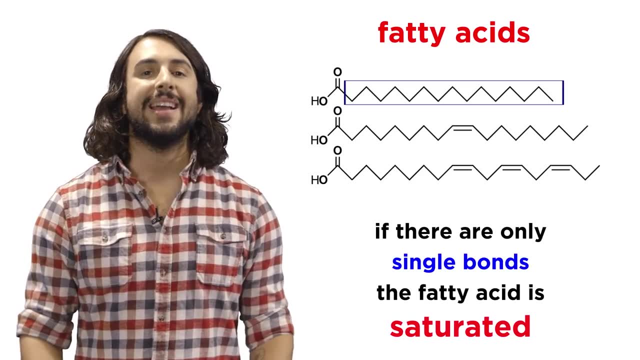 from. Most of the time, lipids are called glycerol. Most of the time, lipids are called glycerol. Most of the time this tail is unbranched and contains an even number of carbons. If it contains all carbon-carbon single bonds, this would be a saturated fatty acid, because 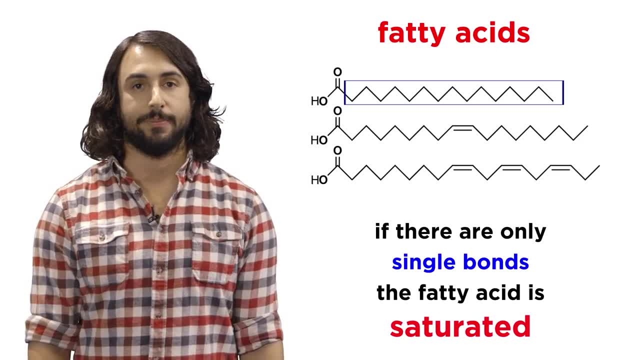 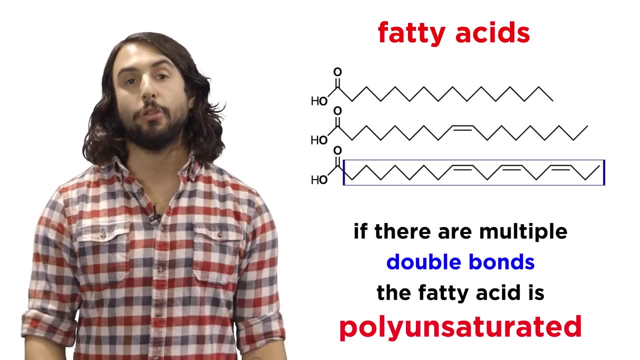 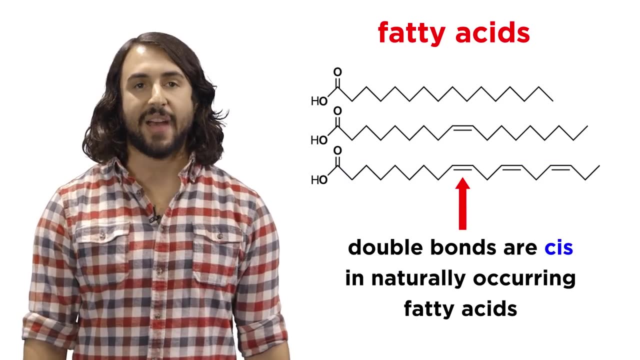 it contains the maximum number of hydrogen atoms possible. If there is a double bond, it's an unsaturated fatty acid. Sometimes there are two or three double bonds, which would make it a polyunsaturated fatty acid. In naturally occurring fats, the double bonds are almost always cis. 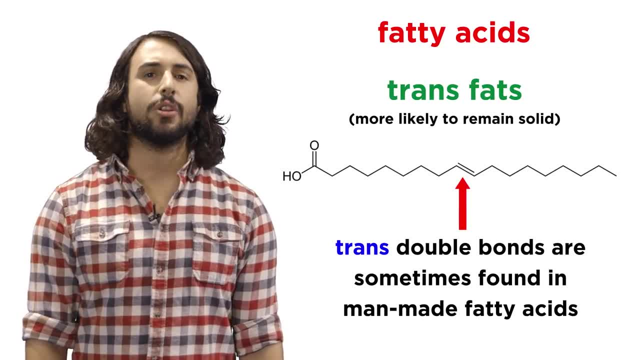 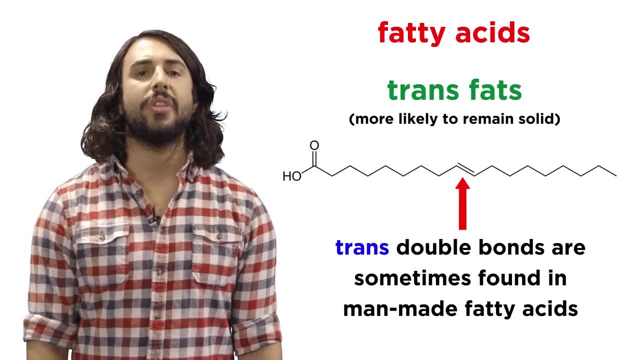 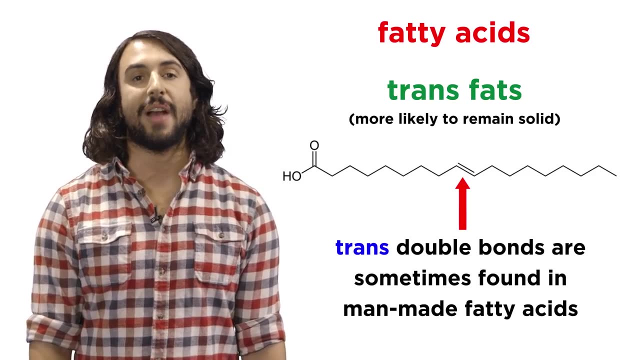 When we hear about trans fats, these are the ones that seem to be harmful to the human body, as their linear shape gives them a higher melting point, so they are more likely to remain solid and more difficult to metabolize. These are associated with cardiovascular disease. 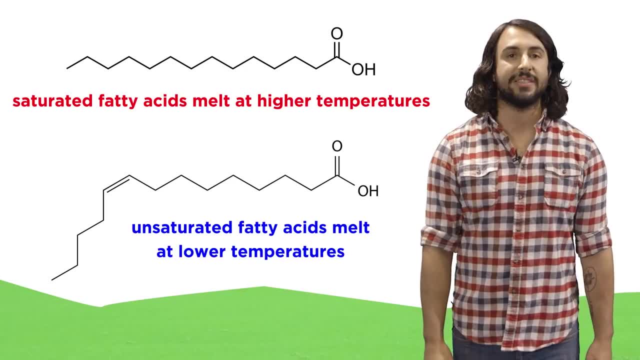 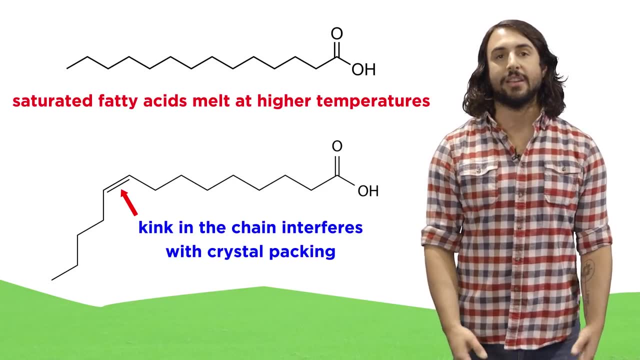 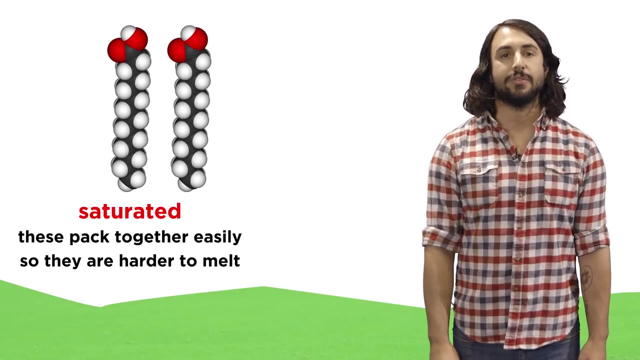 In general, saturated fatty acids have higher melting points than unsaturated ones because the double bonds restrict rotation and therefore cause a kink in the body. It's often a kink in the chain which interferes with crystal packing. Saturated fatty acids can pack neatly and maximize van der Waals' attractions. 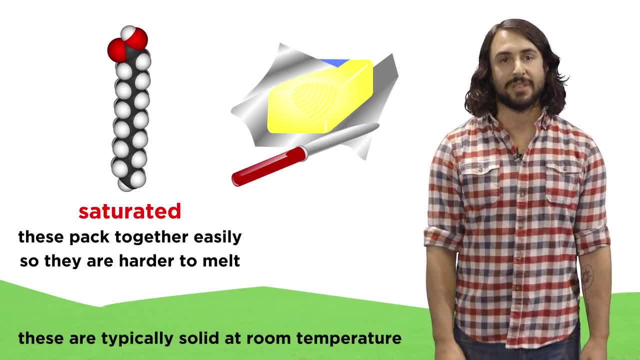 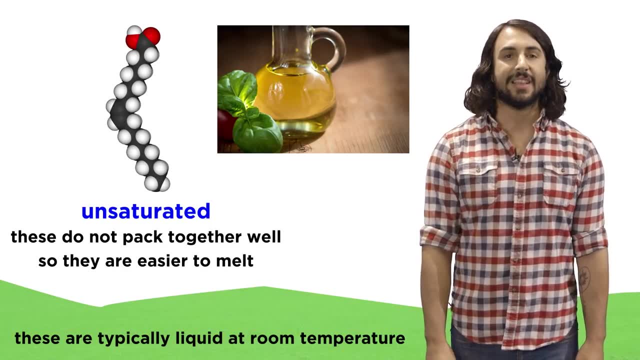 That's why butter which is fully saturated is a solid at room temperature, whereas olive oil, which has a degree of unsaturation in one of its hydrocarbon chains, is less able to form an orderly solid lattice and is therefore a liquid at room temperature. 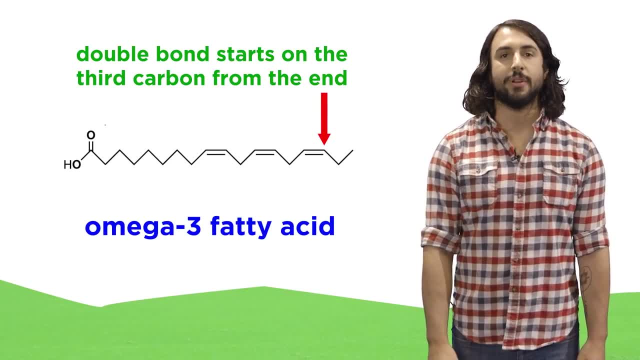 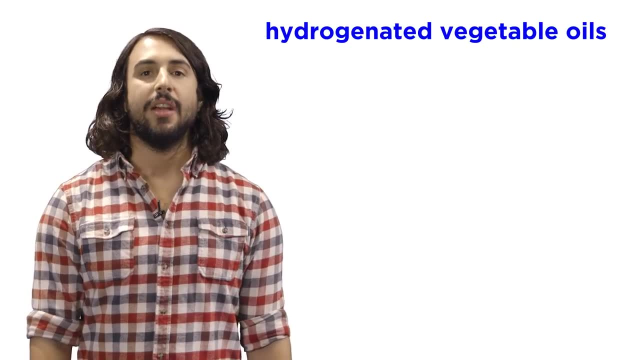 An omega-3 fatty acid is one where the third carbons are more likely to be saturated than unsaturated ones. as they are more likely to be saturated, carbon from the end of the chain is participating in a double bond. when we talk about hydrogenated vegetable oils, these are derived by hydrogenating some. 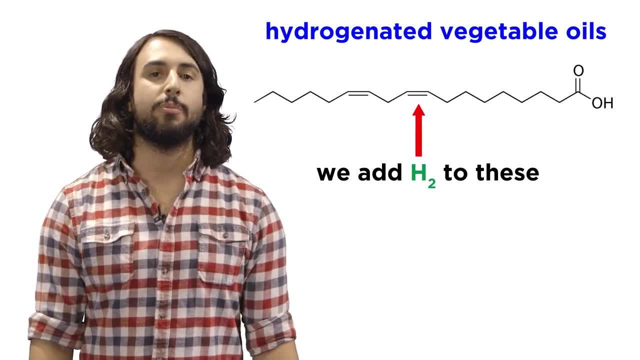 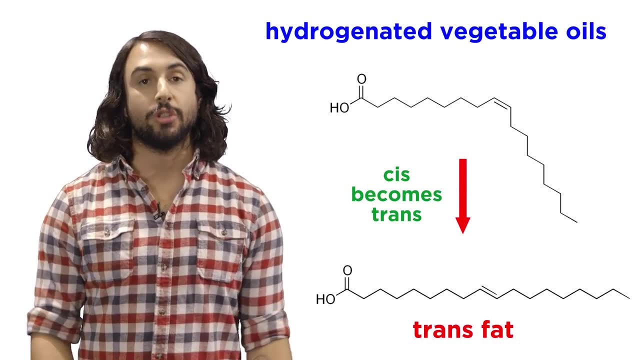 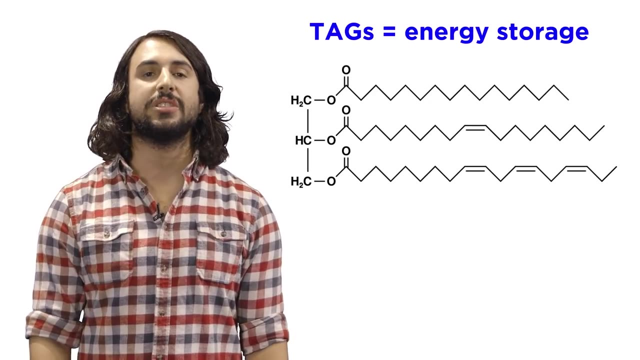 of the double bonds in polyunsaturated fats. one problem with partial hydrogenation is that it can sometimes isomerize double bonds, turning cis into trans, resulting in trans fats which, as we said, should be avoided. in general, fats like tags are used as energy storage when these are metabolized in. 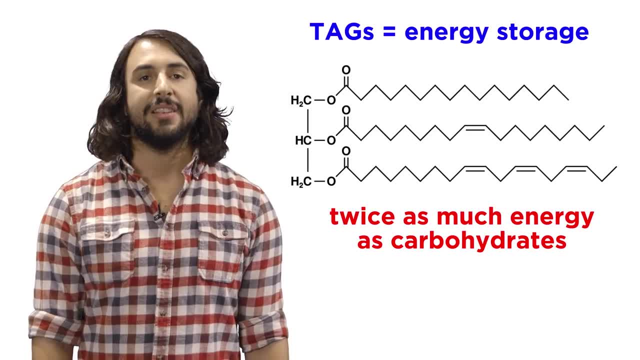 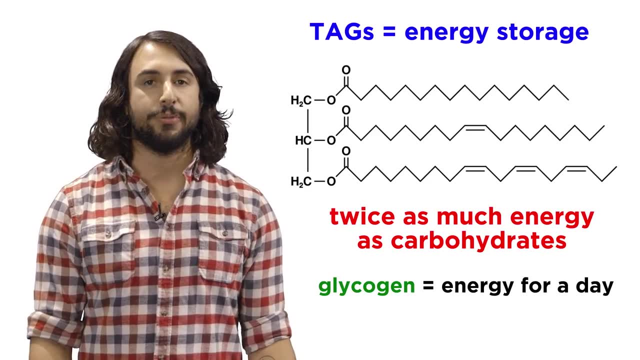 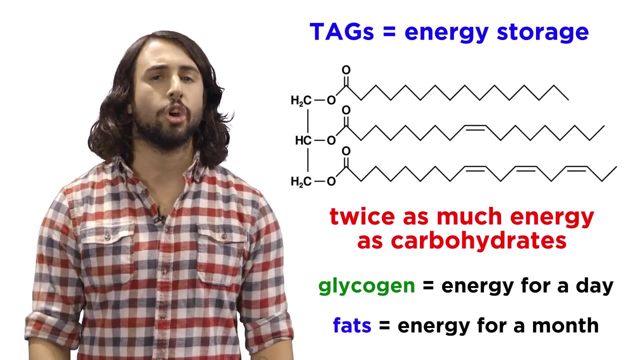 our bodies. they release twice as much energy as carbohydrates, since there are so many carbon-hydrogen bonds. furthermore, polysaccharides, like glycogen, only provide energy for about a day, whereas the fats we store that make up around 20% of our body mass, provide long-term energy storage, which would 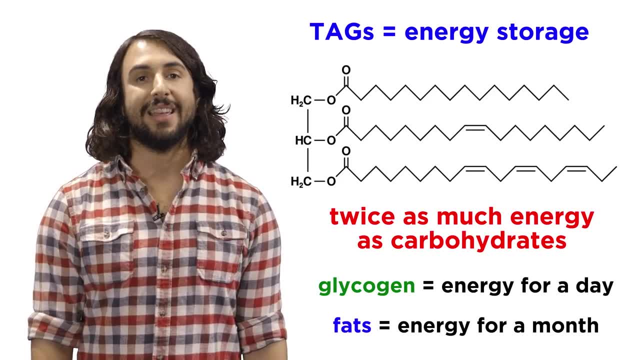 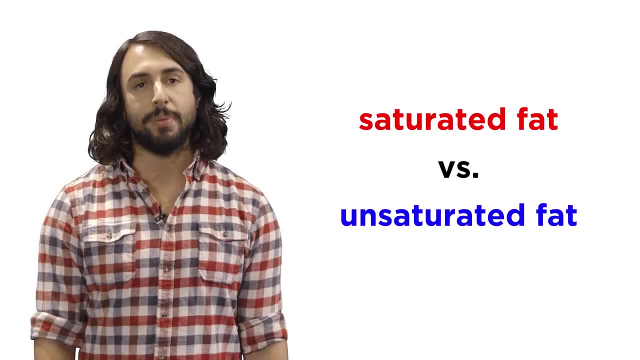 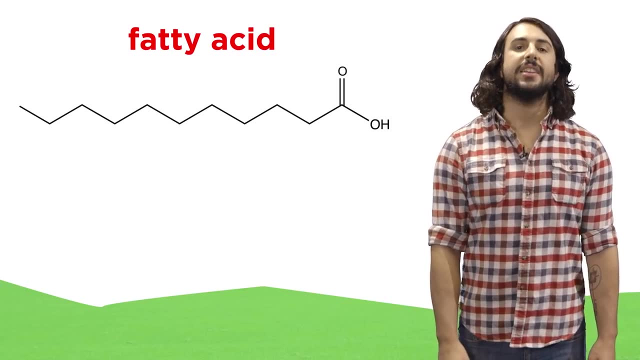 keep us alive for up to a month without any food intake, if necessary. statistically, there is much discussion about how much saturated fat and unsaturated fat should be in our diet, but we will have to examine that another day. another interesting aspect of fatty acids is that, when the carboxyl group is 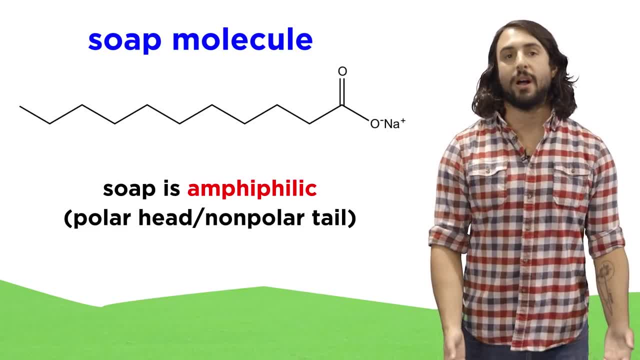 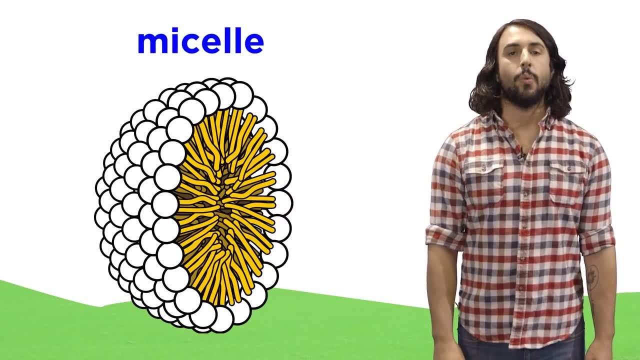 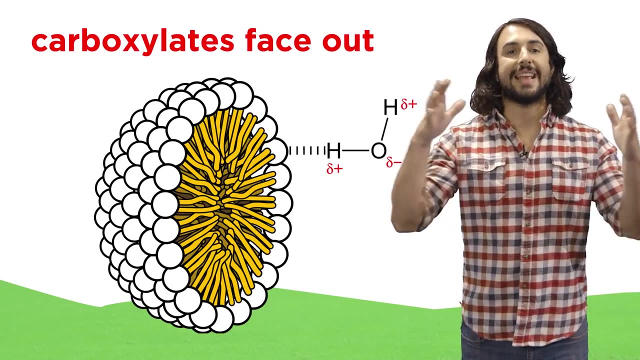 deprotonated to form the sodium salt, you get soap molecules which have a polar head and a nonpolar tail. these work by forming micelles in solution, where many soap molecules orient themselves, with the negatively charged carboxylate groups all facing outwards to maximize ion-dipole interactions with water. 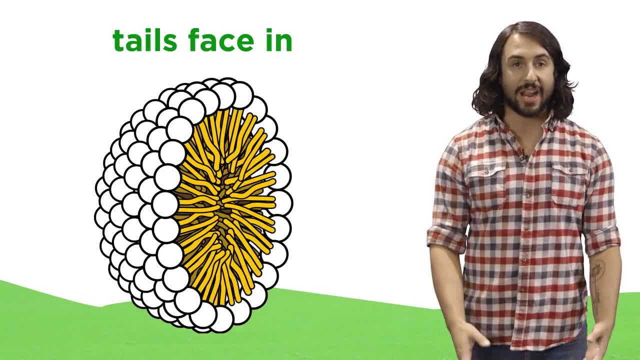 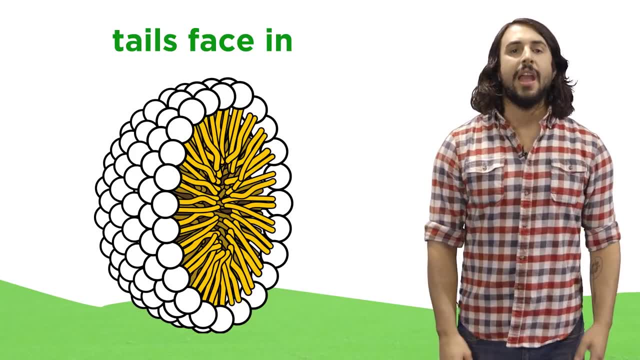 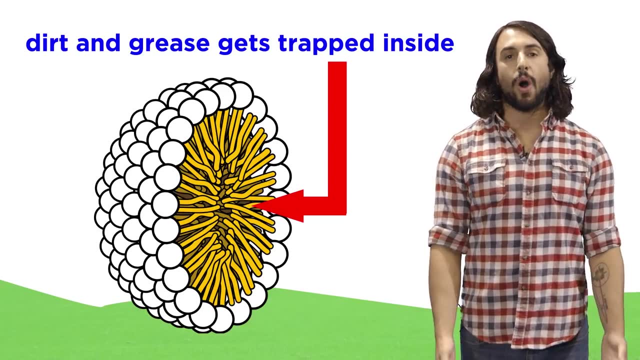 molecules, while the hydrophobic hydrocarbon chains point inwards by exclusion making van der Waals interactions with one another. any nonpolar dirt or grease, which is normally not water-soluble, can get trapped inside and will then wash away with the micelle, which is 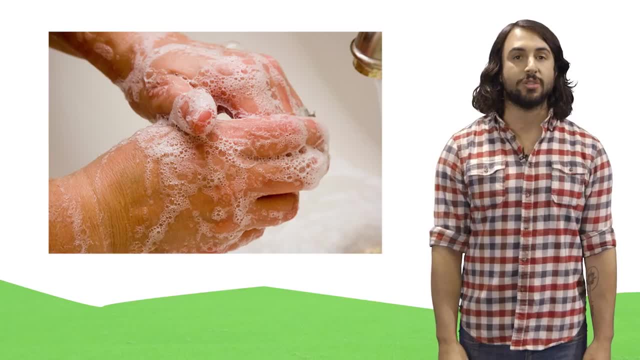 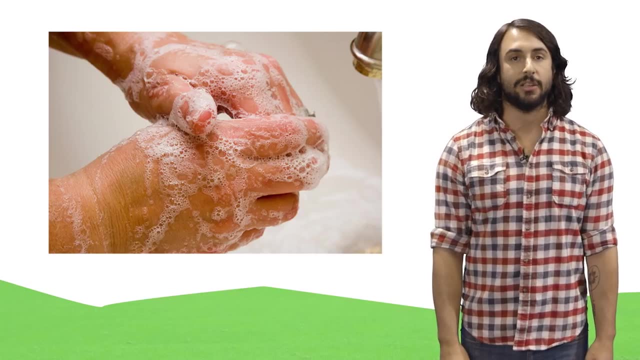 water-soluble. that's why washing your hands with just water alone won't do anything, but add some soap and the dirt gets transported away in little spheres of soap molecules. let's discuss another type of lipid, the terpenes and the. 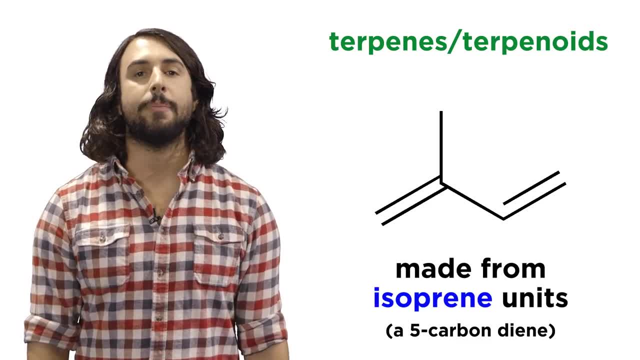 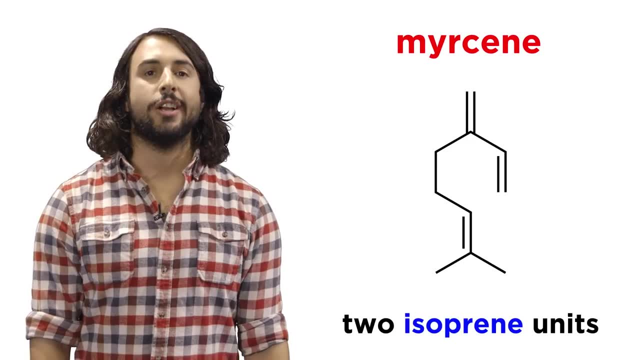 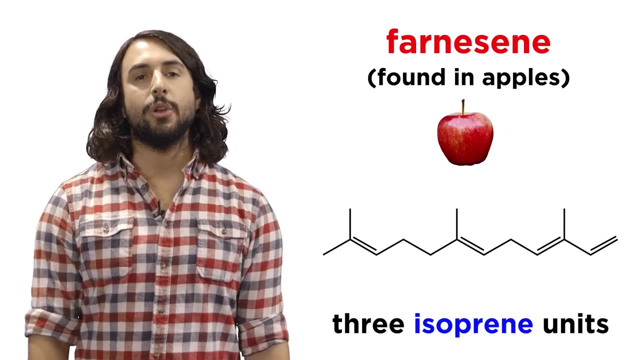 terpenoids. these are polymers made up of repeating isoprene units, which is this 5-carbon diene. here we can see myrcene, a terpene consisting of two isoprene units. farnesine, found in apples, has three. the units can be linked to form. 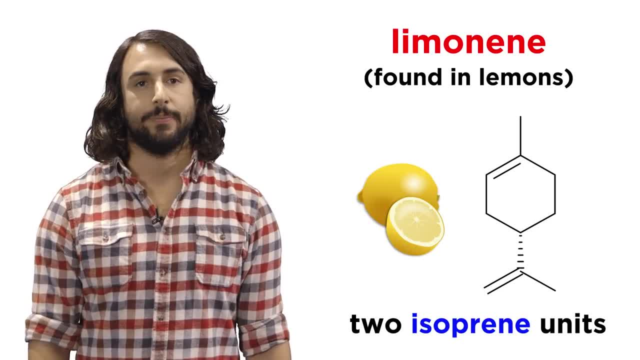 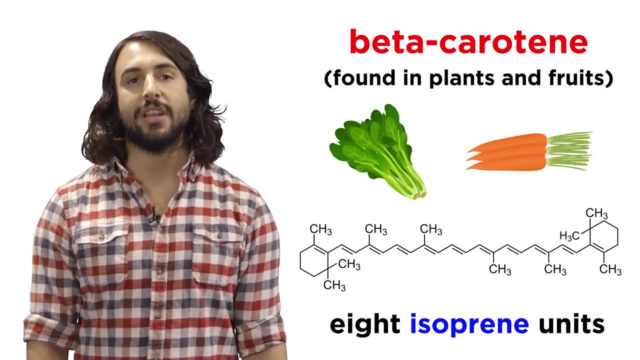 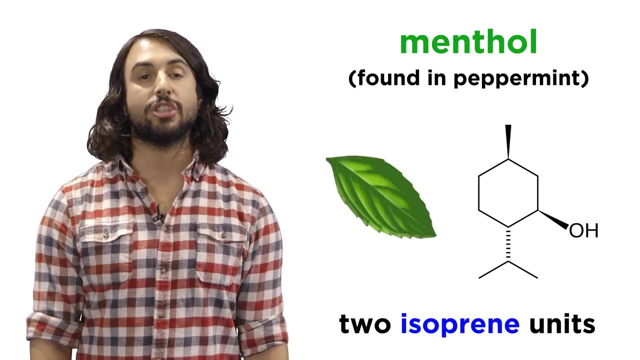 rings, such as in limonene, which is found in lemons. these can get much larger, such as with beta-carotene, comprised of eight isoprene units, which is found in various plants and fruits. terpenoids are similar to terpenes, but they contain oxygen atoms, such as with